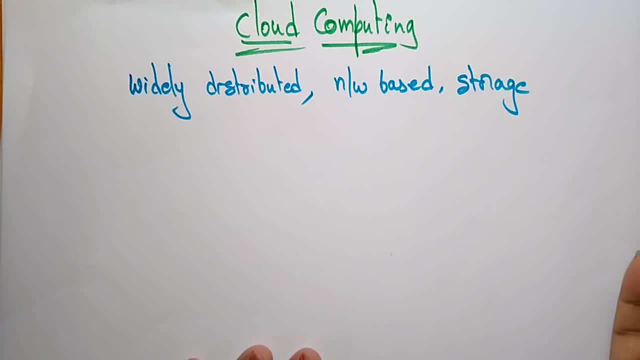 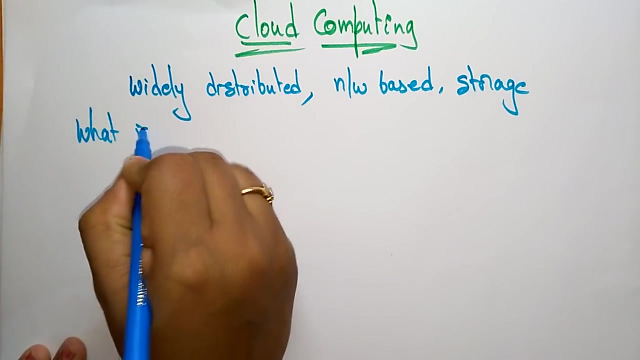 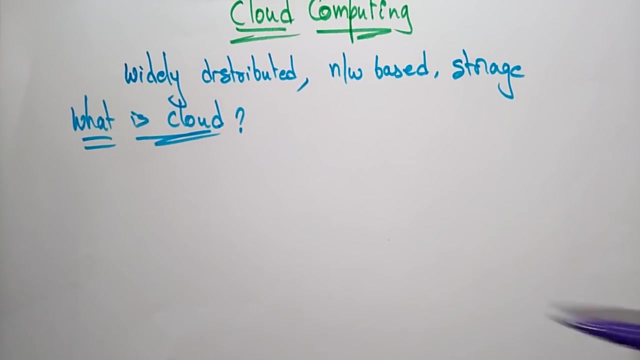 whatever the data that you want to store, you can store it on the cloud. okay, it is a storage and it is a computation. so there are so many definitions, so many terms that are coming from the word cloud computing. so what exactly the cloud? what is cloud? a cloud is nothing but using someone else- server- to host process or 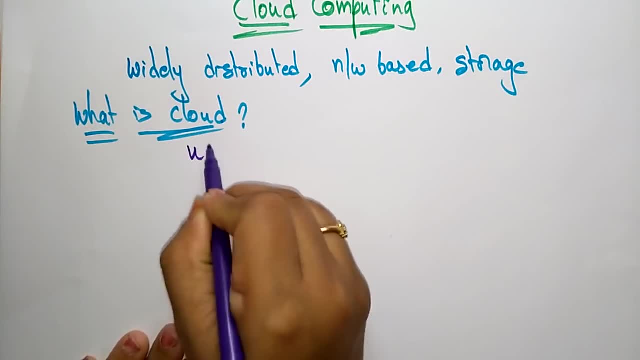 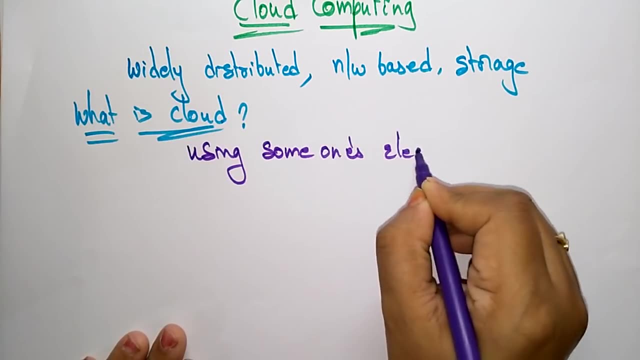 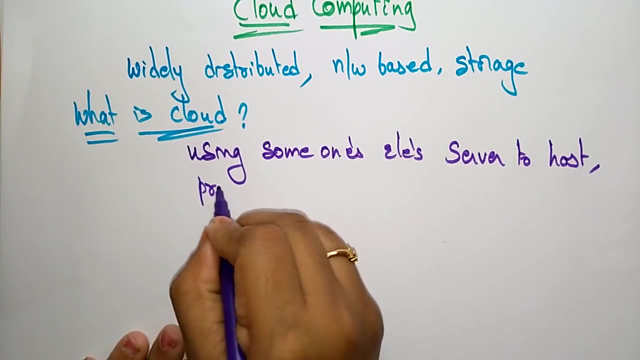 store data. you call it as a cloud. you are just using someone's else server to host, to process or to store data. you are using someone else server. that is a cloud. with the help of the cloud, you are storing the data in, not in, your system. you are not storing your data in your. 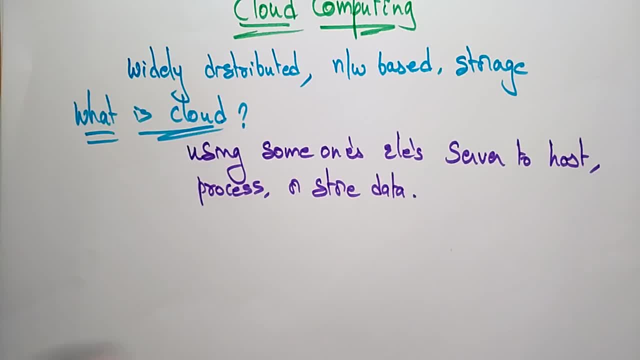 system. if you store your lot of data in your system, your system capacity is very less when compared to the, the cloud- okay. so if you want to store the large amount of data, okay. if you want to store more than the amount, whatever the hard disk you are having, if you want to store that. 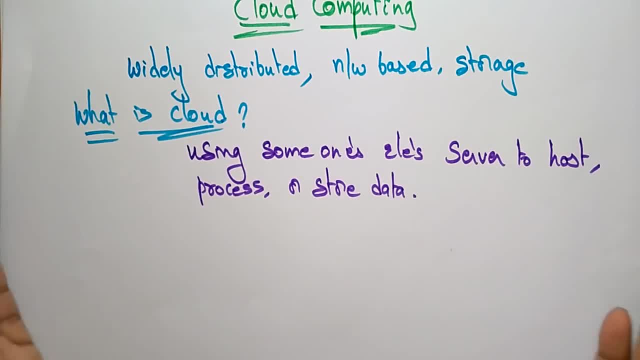 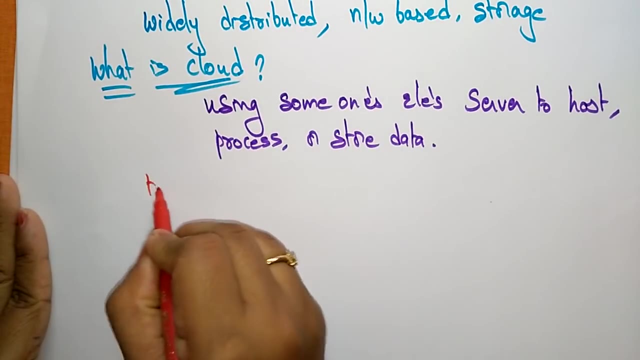 much of amount, amount of data in your system. it is not possible. so then you're for using a cloud, the cloud. a cloud is means using someone else server to host, to process or to store data. let me explain clearly. let's take, uh, if you are using the tablet tab or otherwise, you are using 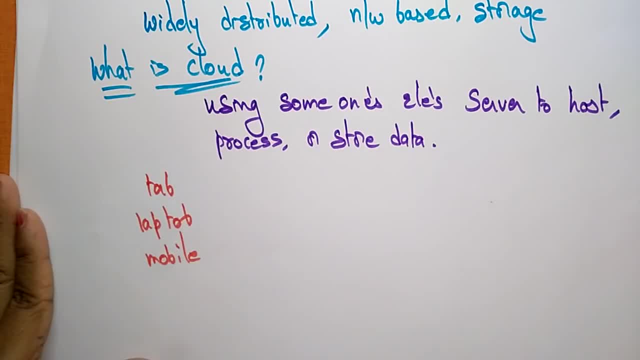 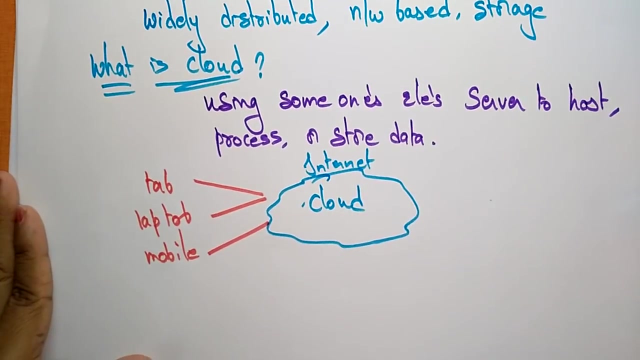 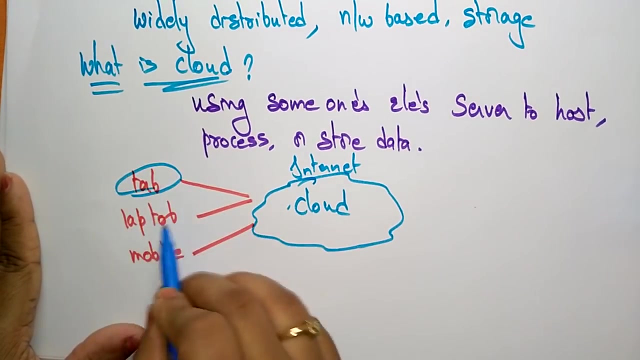 the laptop or using the mobile phone. so these are all the electronic equipments. with the help of these equipments, you are accessing the cloud. this is an internet, or else you call it as an internet. so it's just a cloud. okay, it's a communication internet. so whenever you are accessing on your tablet or in laptop, or you are using the mobile phone, if you, 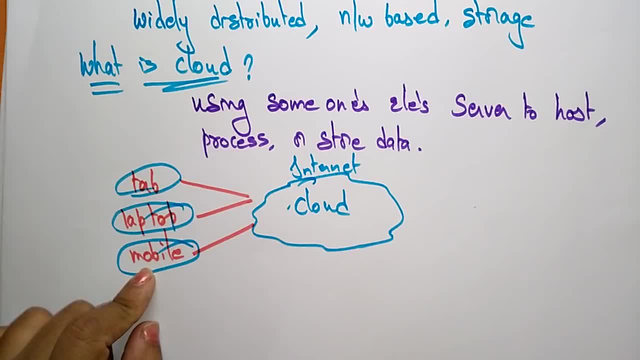 want to access any information. if you want to store any information, okay, let's take if you want to open your mail id. uh, you're accessing your email id. your email id what? whenever you're using the username and password, or you're using the email id, or you can use your email id at any time. 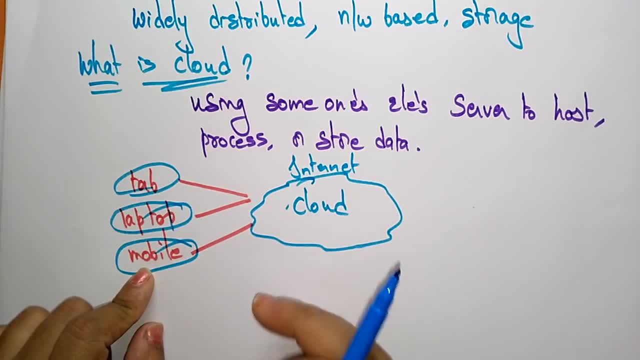 or you can use the email id at any time. your email id is always gonna be your email id. that's what you're automatically. with the help of the username and the password, your link is connected to the cloud and retrieve the data wherever you store. where you stored, you stored in someone else server. 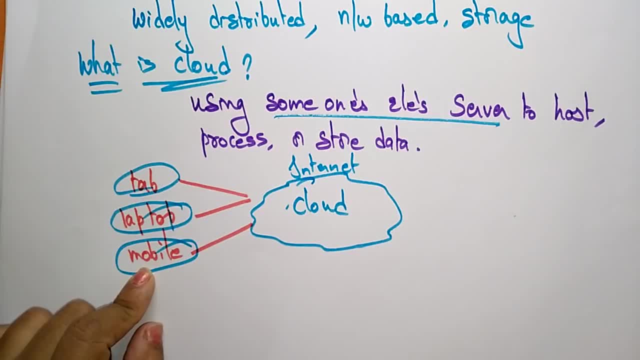 who is that? someone suppose, if you take the gmail in the microsoft server, uh, you are stored. everything the data related to the gmail will stored in the server. okay, so with the help of these microsoft app you're storing, with the help of that server, you're storing your uh files, or? 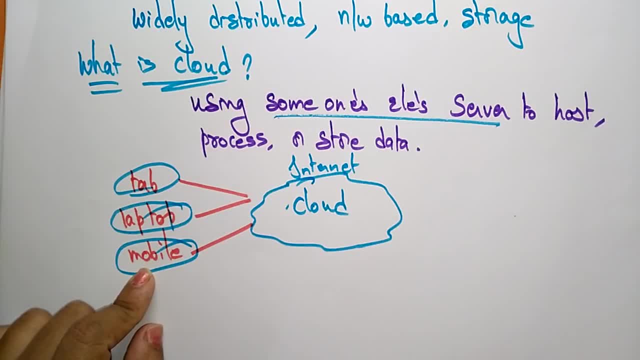 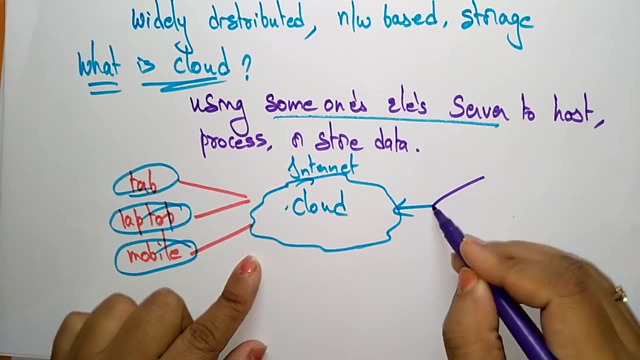 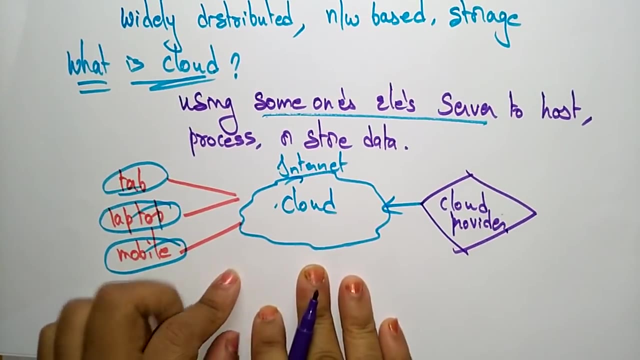 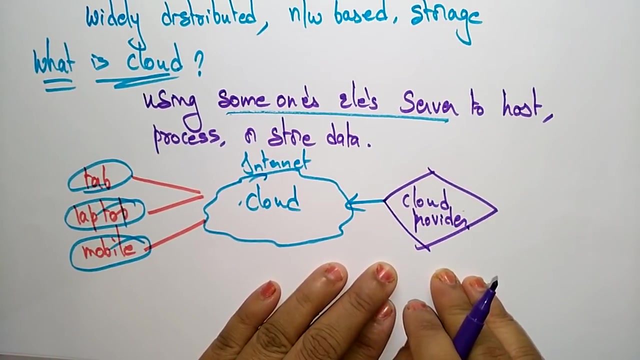 documents or even pictures, whatever it may be, in that someone else server. so this is a cloud, and here you are having some cloud providers. the cloud providers are there. okay, so this is the internet. this internet will be accessing the cloud providers. the cloud providers are nothing but the persons who are. 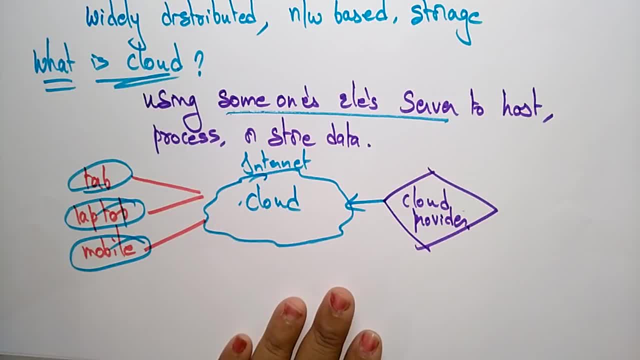 giving the servers means to access to, for storing, for retrieving. so those are the cloud providers. the cloud cloud providers are different people like amazon people, microsoft people, google, so different uh cloud providers are there. they are holding some servers. so in that servers your customer uh relevant information will be stored on that servers. okay, so with the help of the cloud, 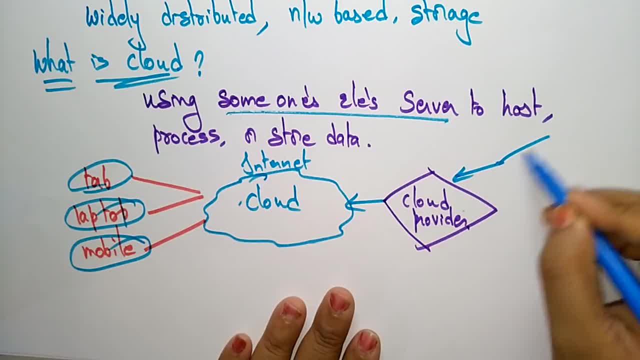 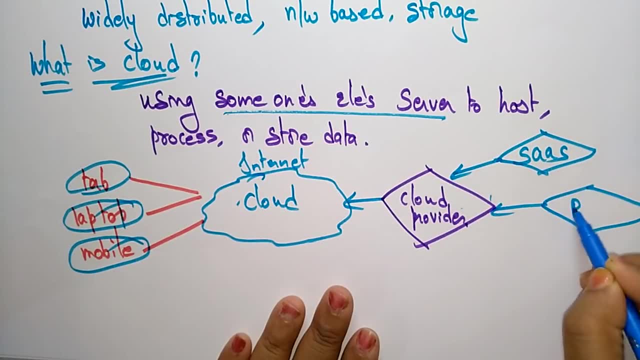 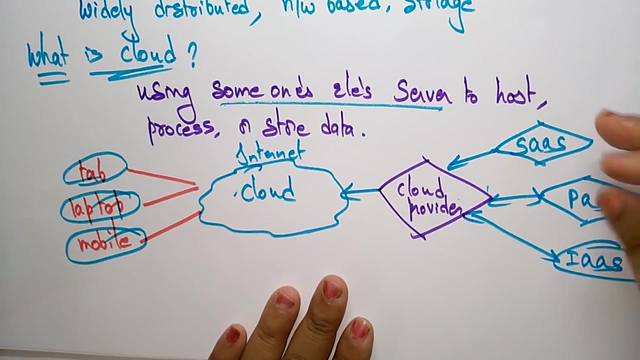 providers. we want to access different services: software as a service, sas, or, if you want, you can access the platform as a service, or else you can access infrastructure as a service. so these are all the services provided by the cloud providers to the customers. so these are the customers, or. 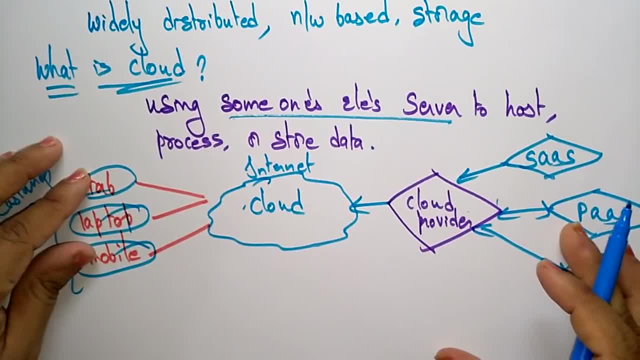 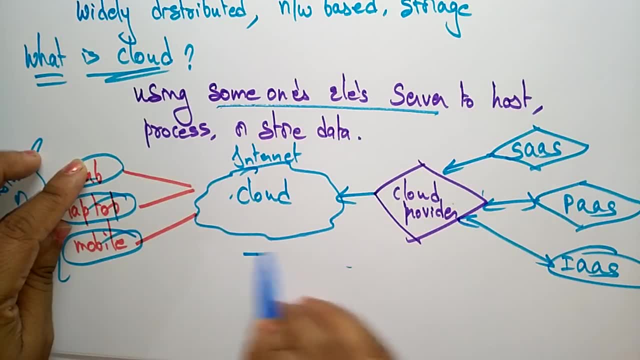 users so they want to use this platform as a service, means the cloud providers, so they- also the user, have caught it for the service, so it is secure. uh, so a page. so when you want to give a service to the users, it is accepted by the network directly for phone or with the authorities or foreign. they are there. it can't support it. 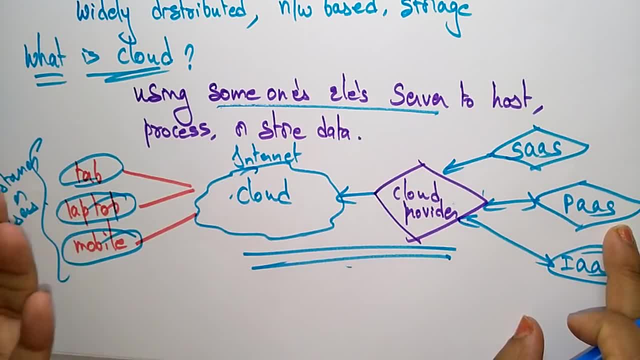 because this is a small amount um, which means so this also applies to um- there are a few nms available. so these customers or users wants to access the software as a service. they want some softwares to. they want to be download, freely download or by paying. okay, so with the help of the